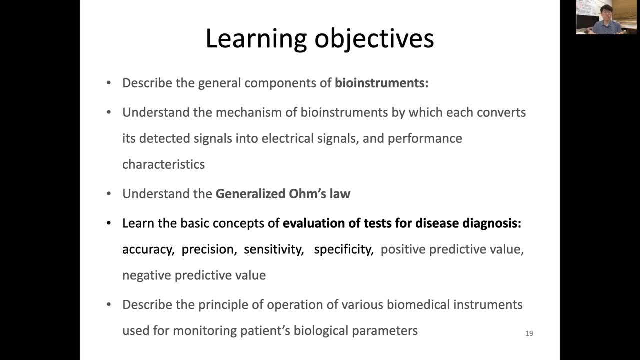 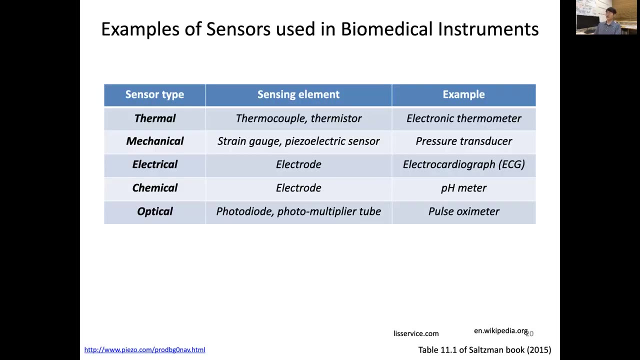 sensitivity and specificity. you have to report to get it approved. So this is a very important concept to know if you want to make your instrument to be able to out in the in the market. So let's first discuss about the sensors are used in biomedical instruments, So there are different kind of sensor types, which is 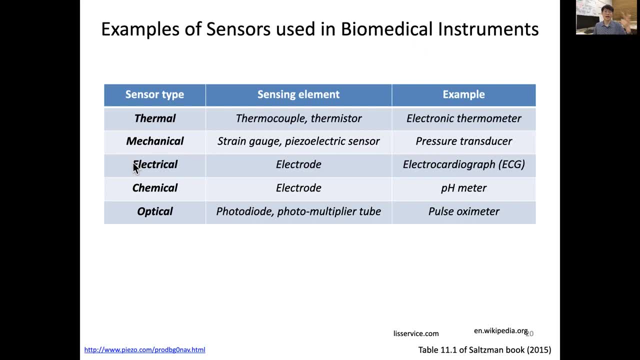 a thermal sensor, mechanical sensor, electrical sensors and chemical sensors and optical sensors. There will be sensing element and I'll give you some examples. So first thermal sensor, The sensing element. you may have heard about thermocouple and also thermistor, So let 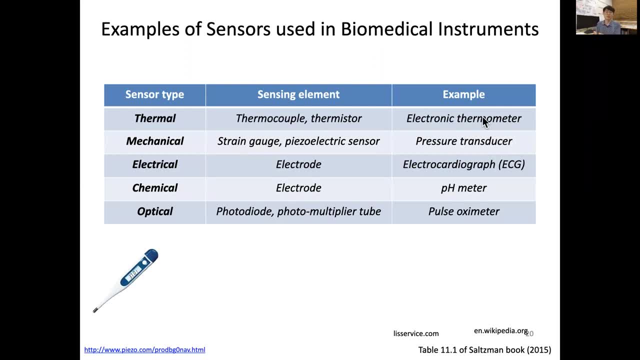 me have an example of electronic thermometer which measures our body temperature. And second, as a mechanic, those sensing elements could involve a strain gauge, which I will discuss further, and or piezoelectric sensor. So piezoelectric is a kind of a displacement, or pressure can give rise to a voltage. 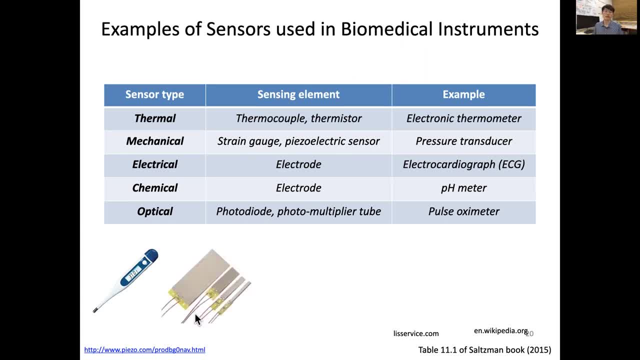 So here's an example as I put this piezoelectric transducer which when we apply a voltage, then this piezo will have a change, So in this case a changing in displacement. So an example as a pressure transducer. one type of pressure transducer I actually use is a piezoelectric. 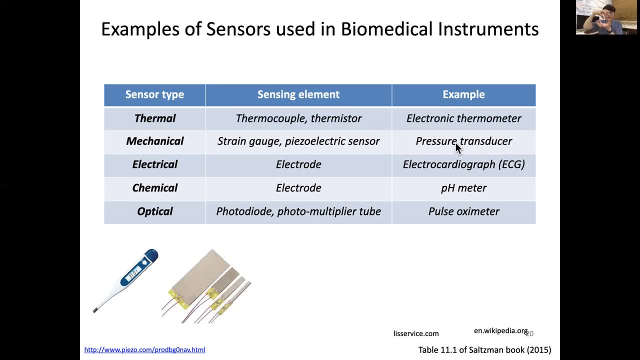 So that we measure, let's say, gas pressure in a specific vessel. There's a specific pressure- So gas- and I want to measure the pressure. We have a piezoelectric transducer that measures this pressure, gives rise to a voltage difference, and that we can measure. 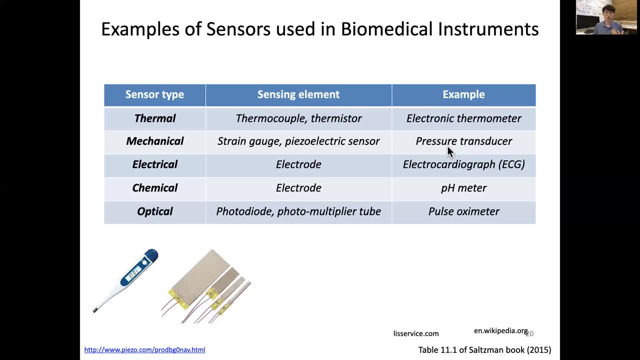 So that's another example of pressure transducer. You see, transduce means converting one type of signal into another form. And thirdly, electrical sensor. one example is electrode, For example, like electrocardiography, and that's like this.